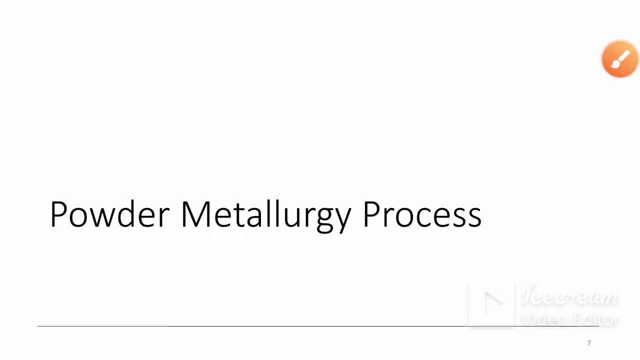 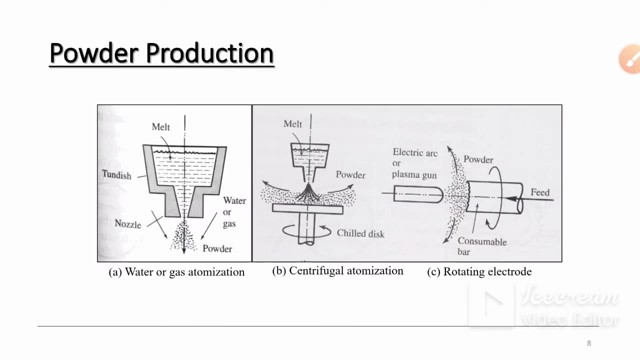 Good morning. The next topic is powder metallurgy process. So first step is powder production. Okay, So, powder production. there are three major methods to produce powder from metal. Okay, So first one is water or gas atomization, Second is centrifugal atomization And third is rotating electrode. Okay, 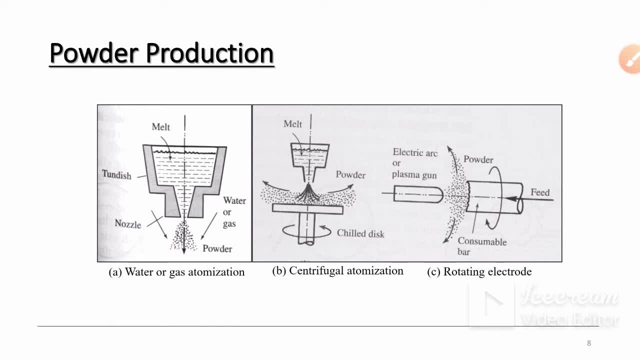 So in first case, water or gas atomization, in which we melt the liquid, we will the metal in liquid form and then we will spray this liquid metal on water jacket or we will spray this liquid metal in air. Okay, So when this liquid metal comes in the contact with water or gas or air, then it gets solidifies at faster rate. 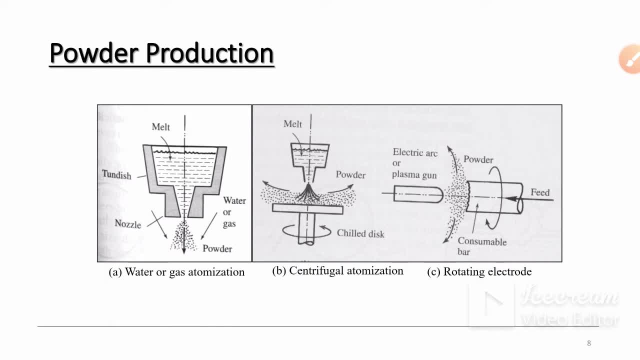 And this spray particles solidifies and we will get a metallic powder. Okay, So how to make powder from metal, solid metal? So first melt the solid metal and pour into the spraying gun and then spray this liquid metal using compressed air and spray in a water jacket or spray in a air. Okay, 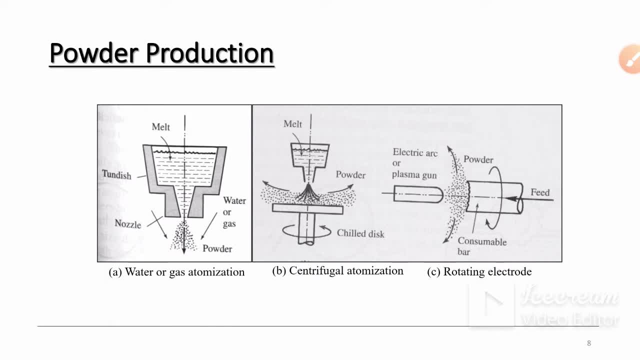 Or gas. So when it comes in the contact with air or gas or water, it will get solidifies and you will get a solid metal particles. So this is first method. Second method is centrifugal atomization, in which we will melt the solid metal and convert it into liquid metal. Okay, And this liquid metal? by centrifugal action, or by rotating at very high speed, this liquid 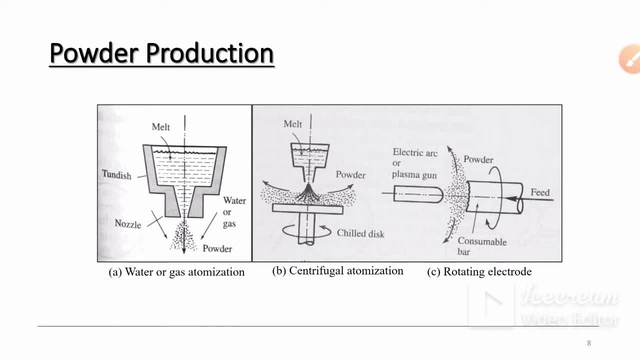 comes outward and we will get solid particles, or solid particles in powder form. okay, the process, only there is a difference of process. so in first case, we will spray the liquid metal in a air or, you know, in a water jacket with the help of compressor, but in second case, we will not using 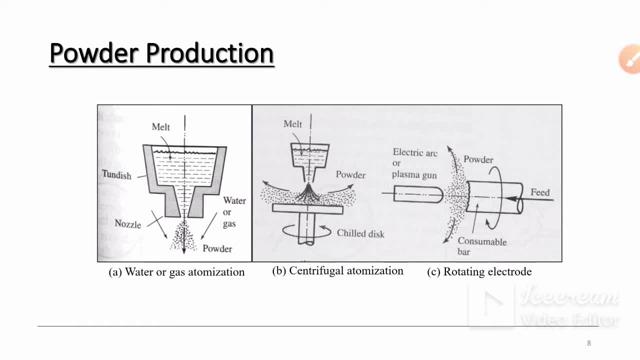 we are not using compressor, okay. we are rotating the object or we are rotating the disk in which liquid metal is there and by this means of this rotation, or rotation very high speed, the liquid particles comes outside this chamber and we will get liquids. is a solid particles or solid part? 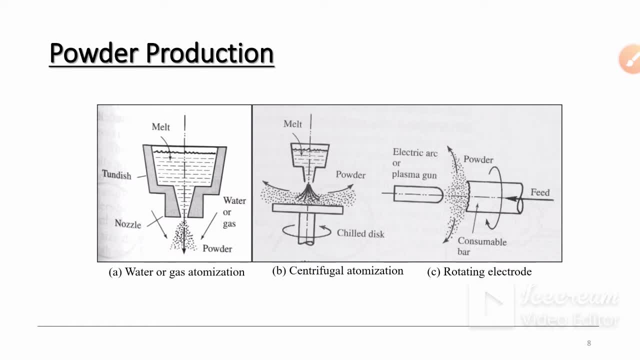 metallic powder at outer side. okay, difference is in method of application- same. third is the rotating electrode. so in third case we are using rotating electrode for creating powder in rotating electrode type. we are using electric arc gun or plasma gun. so the basic function of this electric arc gun or plasma gun to heat the metallic bar. 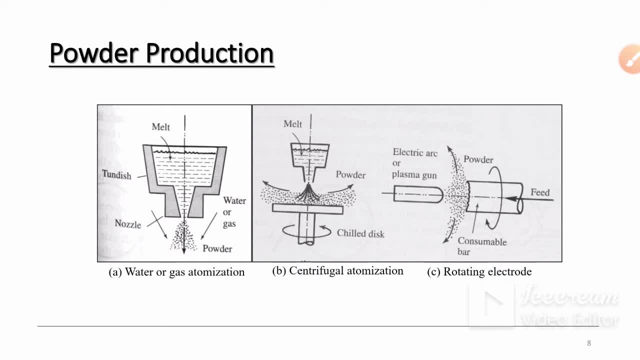 or to heat the consumable bar. okay, so consumable bar is fed against this electric arc or plasma gun and it is also rotated at very high speed. so because of this high speed rotation and because of this hot plasma gun, metal melts and with higher rpm of this consumable bar, the metallic powder or 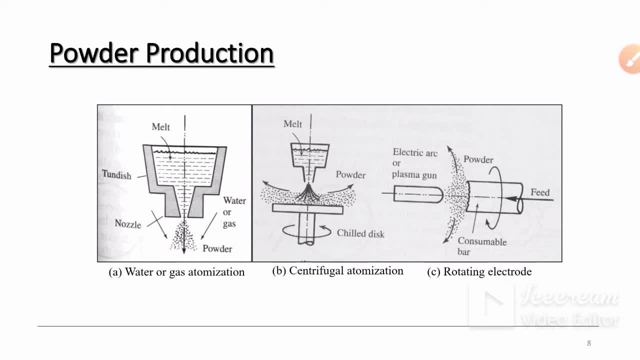 scrap is generated or prepared and which is forcefully collected at outer bin. okay, so this is the basic principle in this powder preparation. a powder production- okay, the third type is near about rotating electrode- is as simple as machining a soft material using hard material. so we are feeding soft material against hard material and with the help of 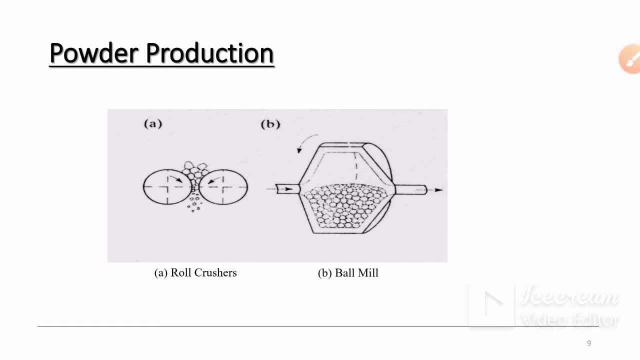 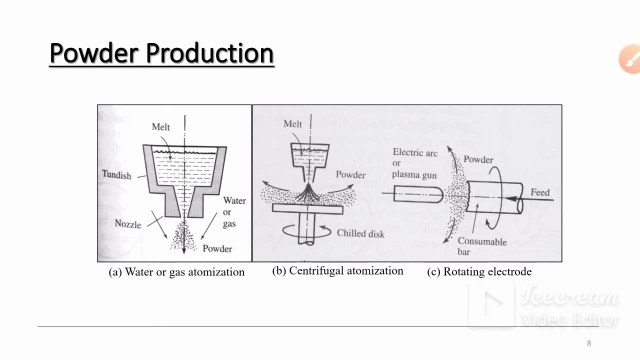 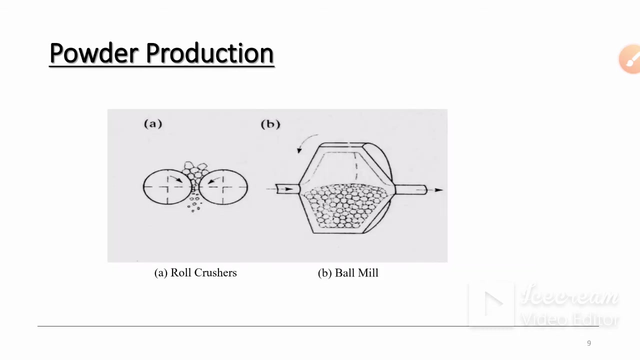 relative moment. we are creating and chips. okay, chips means metallic scrap, part of metal, soft metal. so this in this third type, this is similar to machining, okay, and we are getting chips or micro chips at the end. okay, next processes are roll crushers and ball mills. so roll crushers means there are two. 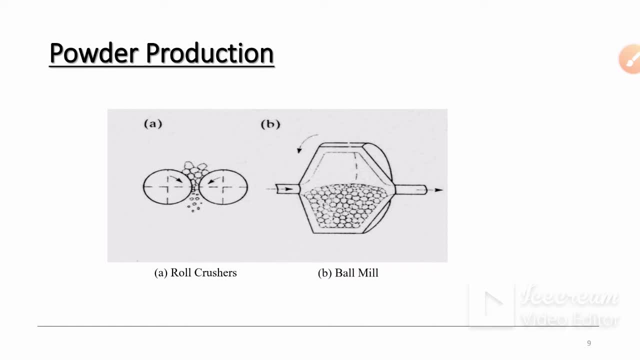 rolls in between, in between these two rolls, we are feeding a metallic objects or metals- okay, and with this crusher, this metal, solid metals, get converted into a solid metallic powder of minimum or less diameter. okay, so using these two rolls, big rolls, or crushers, we crush the metallic stones. 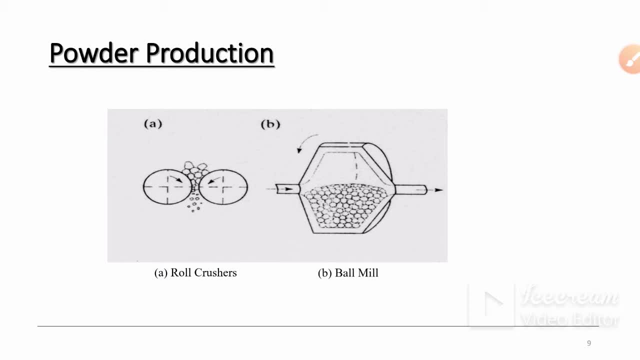 into fine metallic powder. so and next one is ball mill. okay, in ball mill there are some hard material like abrasives are there, and in between, in in this mill we are placing a big stones of metals, okay, and when we rotate this ball mill at higher rpm, okay, or tumbled this mill. then the big grains of metals 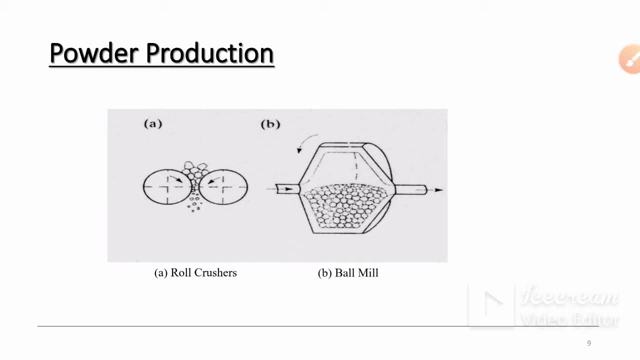 comes in the contact with abrasive particles and there will be a friction or there will be a relative moment between abrasive particles and metallic stones. so because of that relative motion and friction we will get solid metallic powder at the end of this process. so these are some basic techniques to create metallic powder. 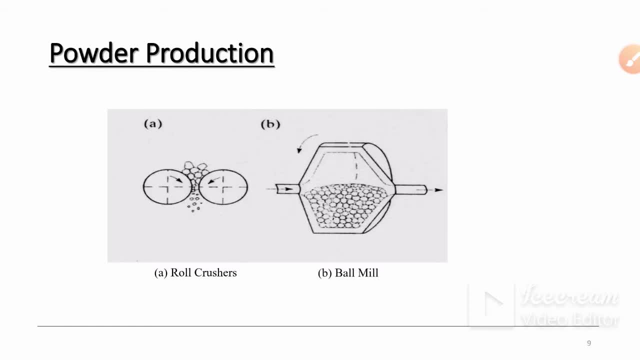 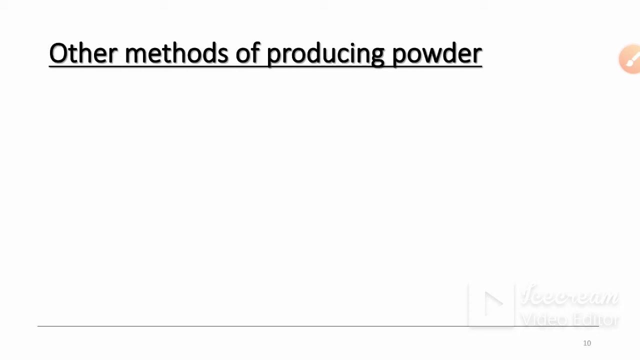 okay, so most common method is using a spray gun. okay, metallic liquid metal is poured in a spray gun and by using this spray- okay, we will get a metallic powder. proteic powder roll crusher is also commonly used. okay, so these are some methods of powder preparation. some other methods of powder preparation are: 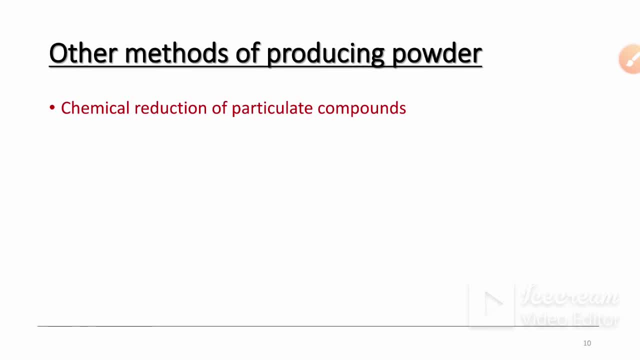 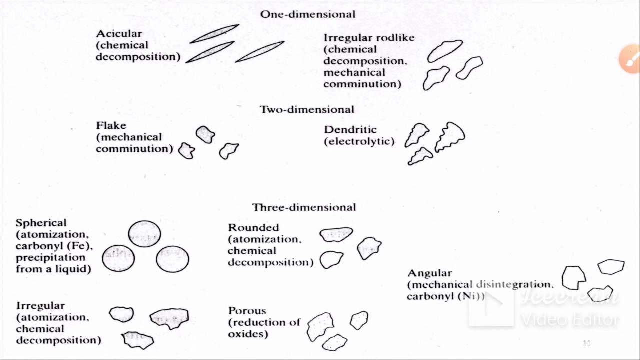 chemical reduction of particular particulate component compound, then electrolytic deposition, then pulverization or grinding of brittle materials, then thermal decomposition, then precipitation from solution, then condensation of metal wafers. so these are some commonly used techniques or methods to produce powder. okay, next one is powder particles. so how powder? 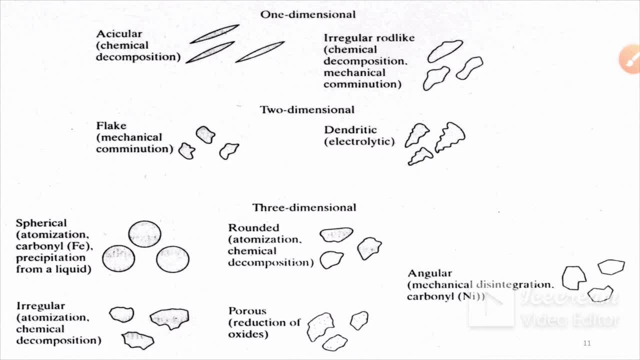 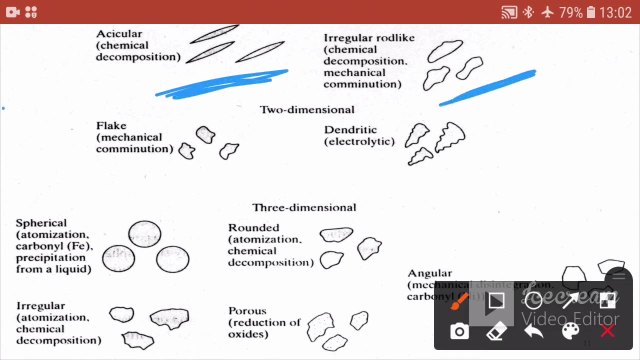 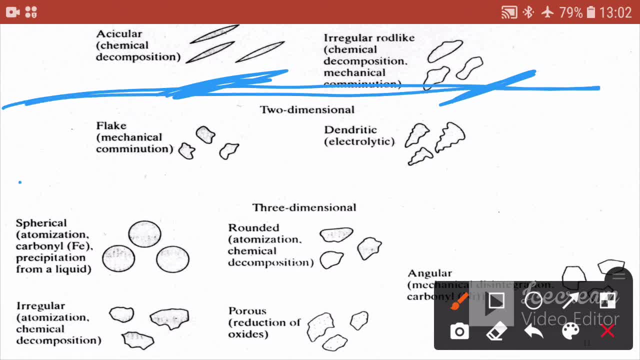 in one dimension. okay, only one dimension is there and the length is there. next, two dimension. in two dimension we will have a surface area. okay. so flake like or dendritic like particles are found. okay, in this two-dimensional type and in three-dimensional you can have. 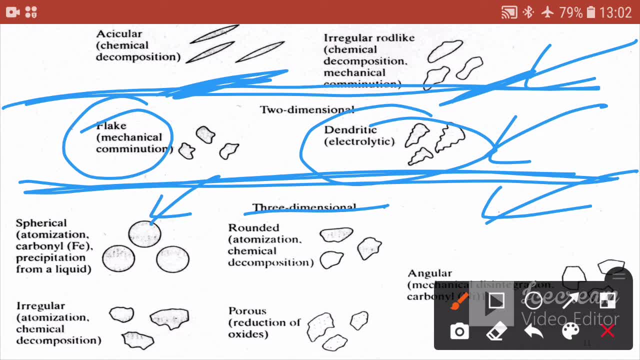 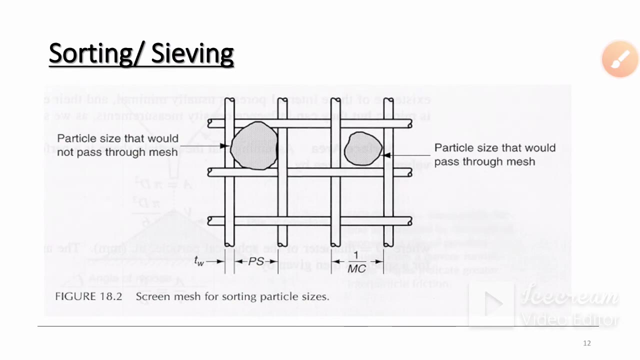 surface area plus thickness. okay, surface area plus thickness, spherical, which is less commonly found, so rounded it is more commonly found and thus irregular. is there? then porous there? angular is there. so there are number of size and shapes of particles. okay, next step is sorting or sieving. 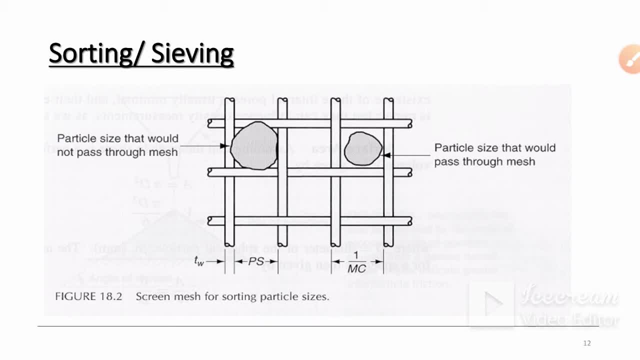 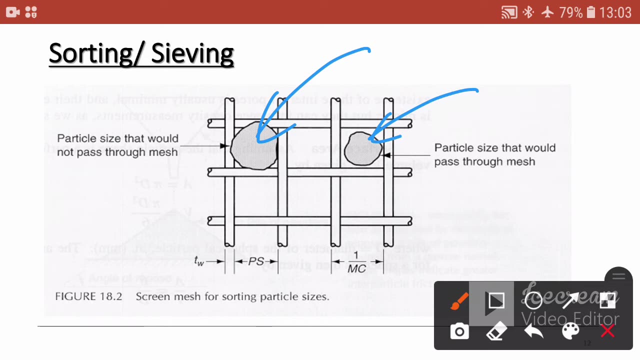 so first step is powder. preparation is over now. how to do it, how to sieve or how to sort the particles: okay, so there is a grains. okay, there is a grains- bigger grains, smaller grains- when we prepare a particles or powder, okay, so to sort different grains, we will. 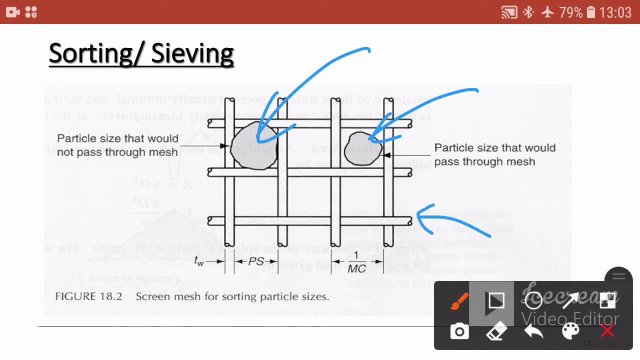 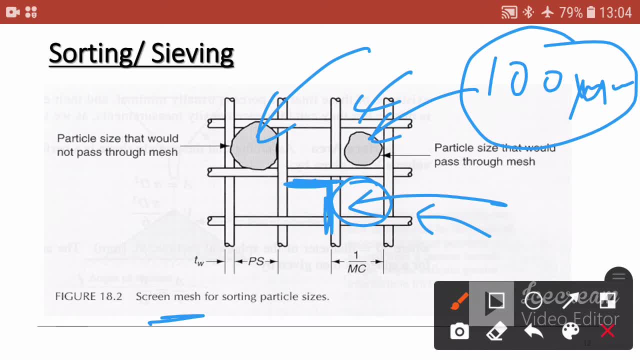 diameter. say it is length and width, 100, 100 okay, or 101 or 101, okay. when we keep 101, 101, then less than 101 will pass from this, okay, and more than or bigger than 101 micrometer diameter will be on these helps him or on the mesh: okay, they will not entered in the from the this mesh. 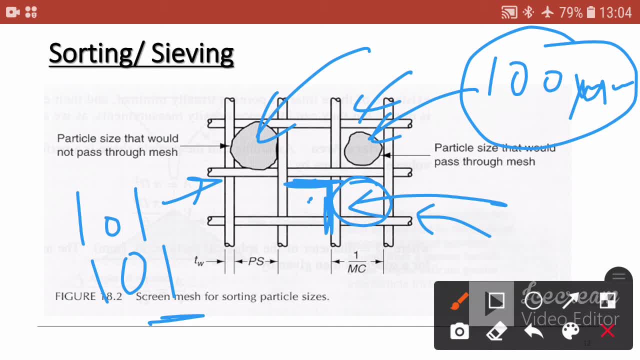 okay, they will be on the mesh or on the céu only. okay, so by this way you can classify or you can salt the particles. okay, so small diameter part ikal will enter from the si or Mesh and bigger particles will be on the C and large particles will be enter the C or are mesh and we will see. 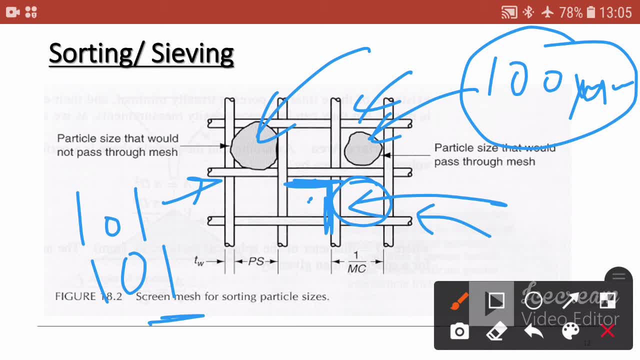 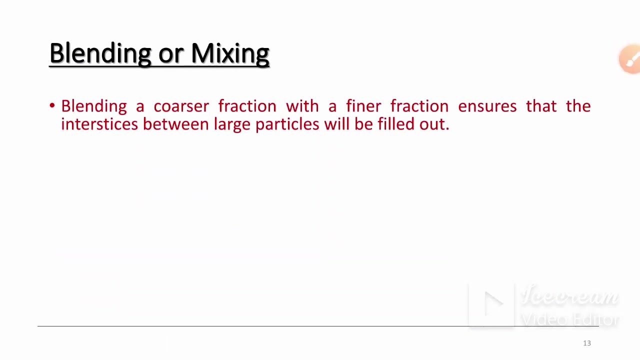 the sieve only. okay. then you need to again crush or again prepare powder from this bigger grains. okay, so this is next process: sorting or sieving. next is blending or mixing. so this is next process, in which blenders- sorry, binders- and additives are added. okay, so blending a coarser fraction. 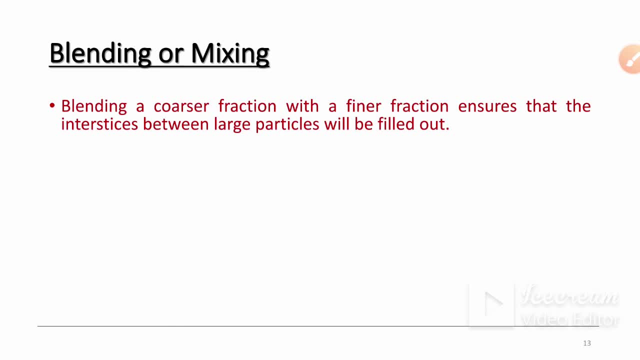 with finer fraction ensures that the interstices between large particle will be filled out. so powder of different metals and other part materials may be mixed in the order to impact special physical and mechanical properties through metallic alloying elements. okay, so mostly copper ion are added, which creates stronger bonding between different different particles. okay. 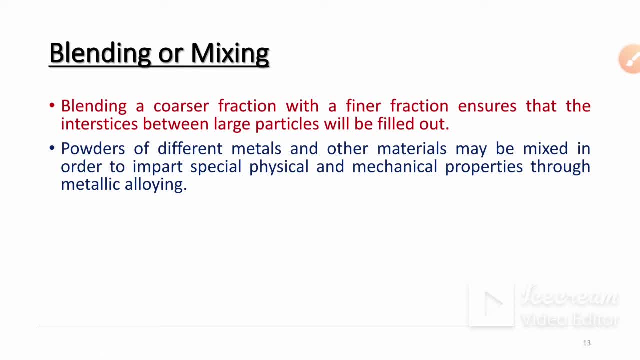 sometimes wax, sometimes other plastic or other. any materials are added to create a stronger bonding between all the particles, so lubricant may be mixed to improve the powders. flow characteristics: okay. some lubricants, such as oil, wax- okay. are added to create or to make material or to improve the materials characteristics. next, binders such as wax or thermoplastic polymers are: 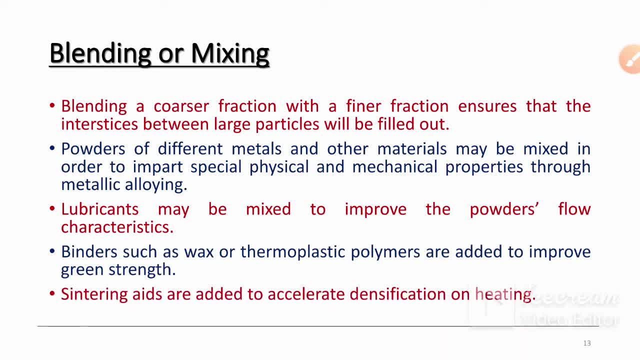 added to improve the green strength sintering aids, to add accelerate densification on heating: okay, we will see this in next slides. okay, so binders and additives are mostly added to improve the mechanical, physical properties of metal and also to create a stronger bond between all the 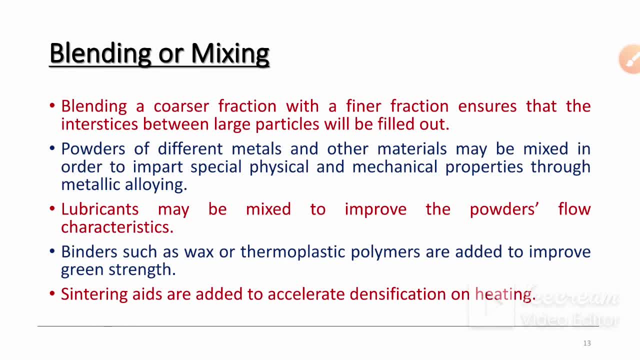 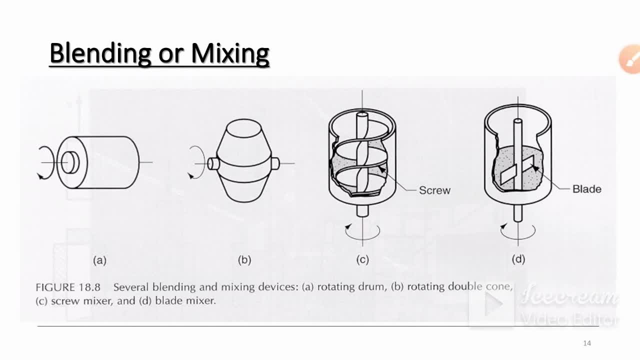 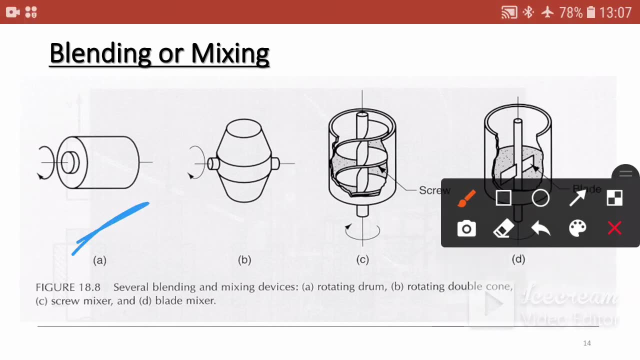 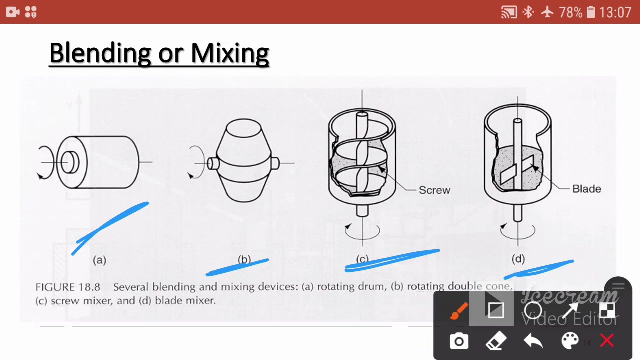 particles present here. this is next step, so several blending or mixing devices. so first one is a rotating drum, second one is- this is rotating term, okay. second one is rotating double cool mixer. and fourth one is blade mixer- okay, so these are the four different methods used to make proper dough, okay. so first we will add our metallic powder in this. 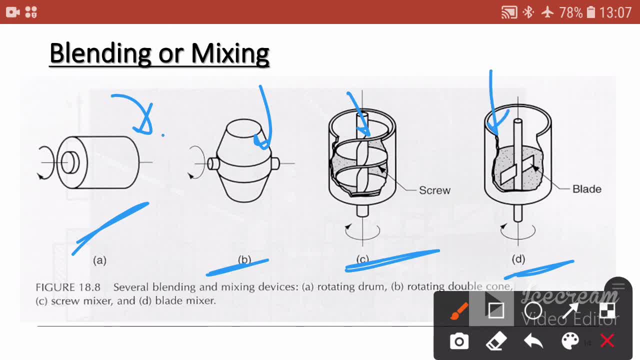 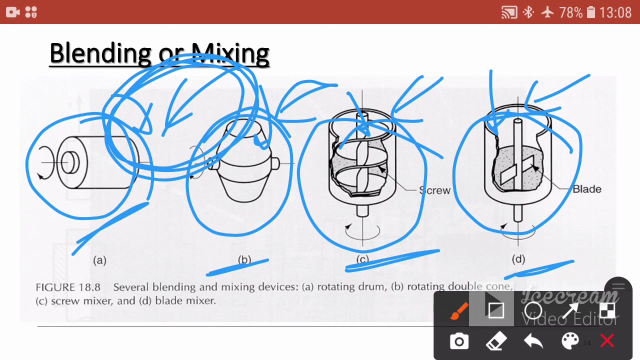 chamber, okay, any chamber, and then we will add some binders and additives there, okay, so after addition of all these, we will then move, or rotate, okay, all these mechanisms. so by this rotation of this mechanism, what will happen? this: two metals, metallic powder and additives or bend blenders, mixed well, okay, or? 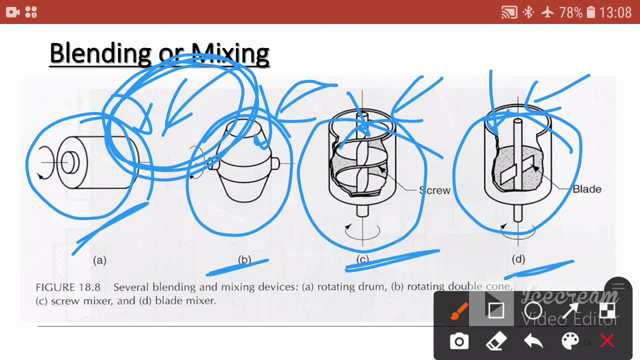 mixed properly. so, after proper mixing, then we will create a dough of this mixture and we will place this mixture in this chamber and then we will add this mixtures dough in a die okay, or on a die okay- upper die or lower die, and then we will use our mechanical, hydraulic or pneumatic press to compress. 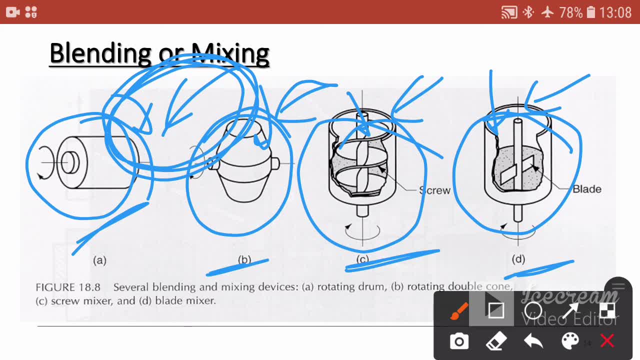 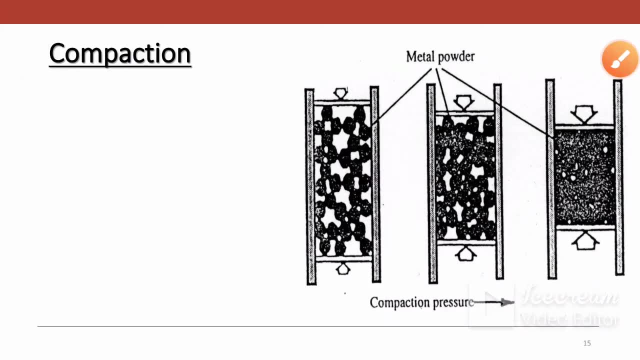 this mixture okay, and after compression we will heat this mixture. okay. so next step is compression or compaction. so this is next step: blending, mixing. next is compaction. so in compaction we will place, for example, there are metallic powder plus adders and binders, so we have placed our mixture here in between. 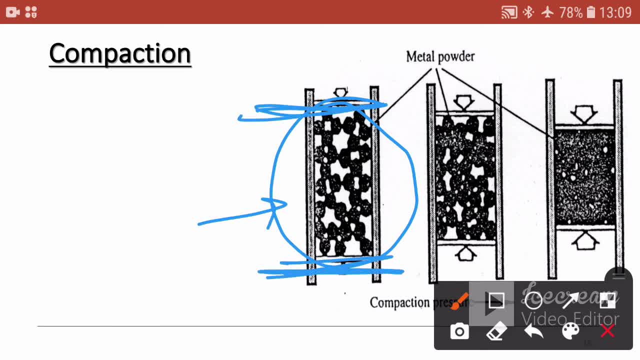 lower die. this is a lower die and this is upper die, between lower die and upper die, so lower die. I have fixed the lower die. or you can move both the dies, okay. so in this case we have moved the both the dies. here we have moved this die and because of this, 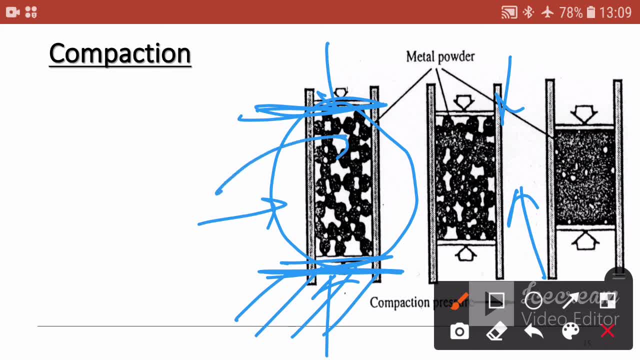 moment, you can see the void space between these particles. so there is a void space. if you see here, if you see in between those, these two, there is a void space. there is a blank space, there is white space. okay, so reduce the white space we have in, increase the pressure in between this. 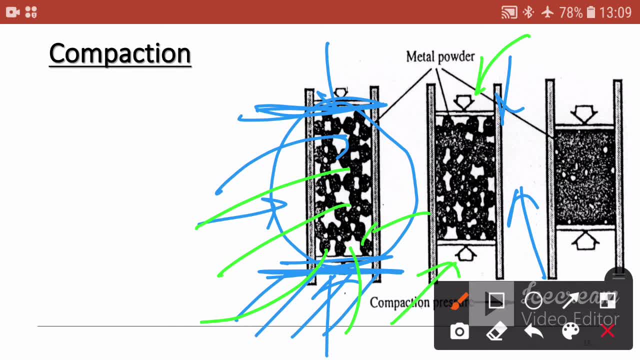 die. so because of that higher pressure, you can see, the gases between or the free air between these particles will be removed and we again compressed here. okay, so by this compression you can see there is a negligible, very little void space is there. so because of that white spread, 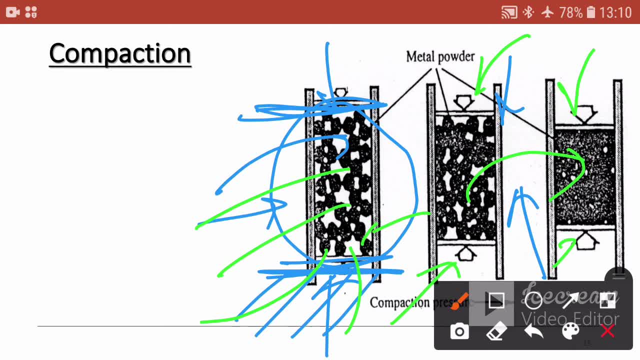 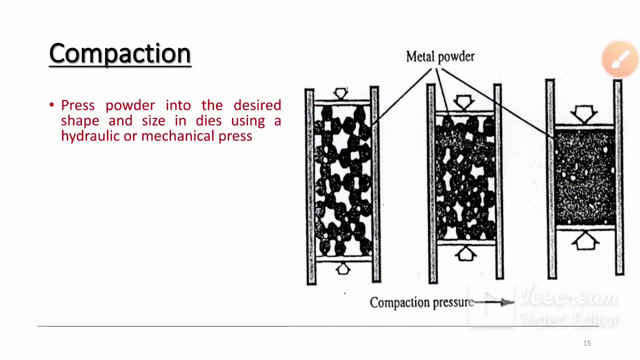 there is a porous material. okay. so because of that, this voice void space only material gets, or material is porous. so this is compaction process. so press powder into a desired shape and size in a dice using hydraulic or mechanical press. then pressed powder is known as green compact. then cold compaction is with 100 to 900 mpa. 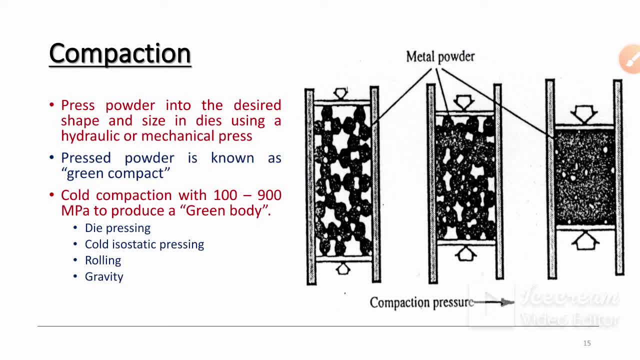 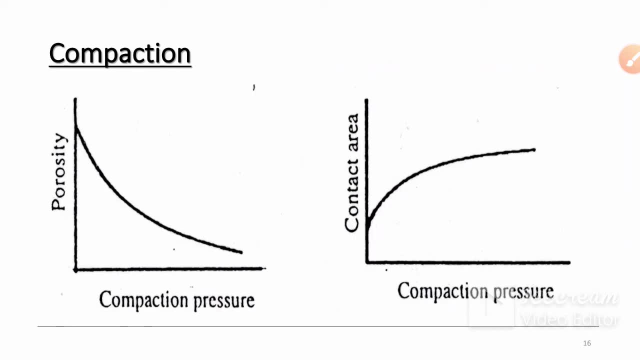 megapascal to produce green body. so type processing, cold isostatic pressing, rolling and gravity are the methods. then injection molding- small or complex part- so induction molding is also one of the process- is used to compact or press the material. okay, this is compaction, so you can. 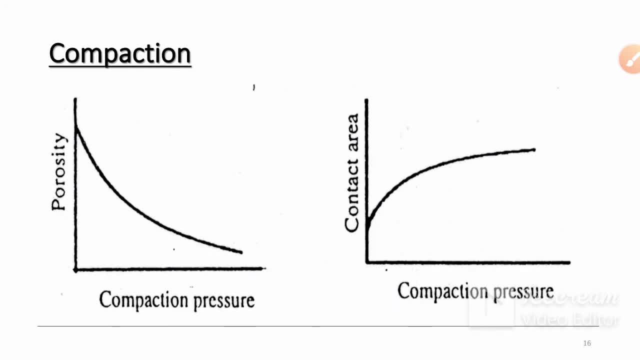 see, the porosity reduces when we increase the pressure. okay, porosity means number of holes of pores in a material. okay, when we compress at very high pressure, then the holes diameter reduces. okay, porous hole diameter reduces or will. be negligible means no diameter, will no uh spaces. 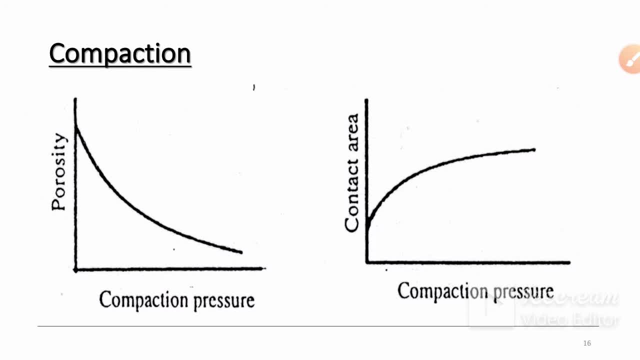 will be there, okay, when we increase the pressure of this lower and upper die in between this lower and upper die, so more material get compressed. and we will get compressed material- okay, with minimum porosity or minimum holes or minimum void species, so as material is more porous. 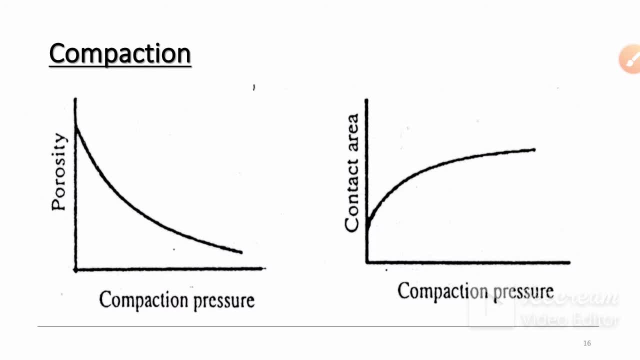 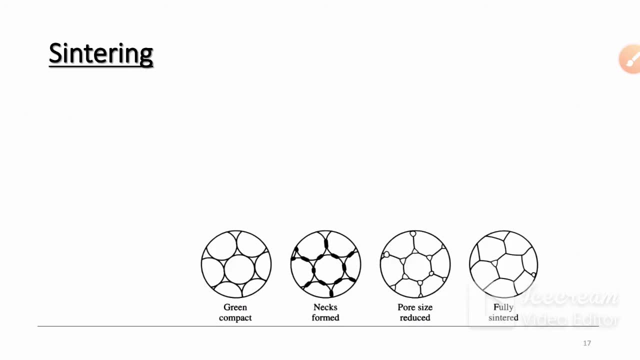 there is a tendency to scattered it out means particles will scattered when balls means brittle neutral, so they are. next is sintering. so sintering is nothing but a heating, but in this heating process there is no oxygen present, or negligible oxygen present. okay, so why there is no oxygen? 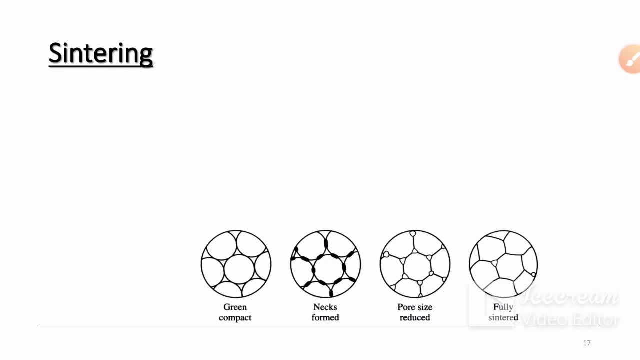 when we heat the metal because of that oxygen material gets, or material will the tendency of, it will burn. okay, so there should not be any burning there. okay, to avoid the burning, we are not using oxygen or we are not heating in presence of oxygen. so by heating what will happen? this you 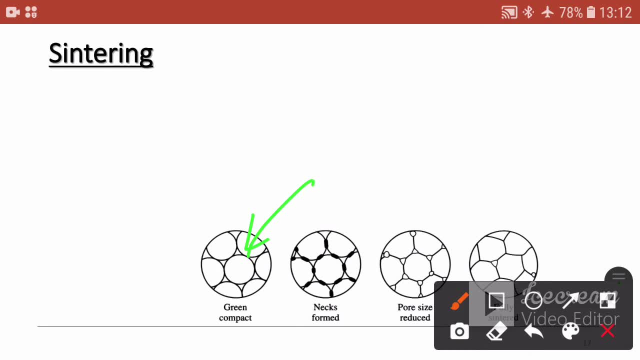 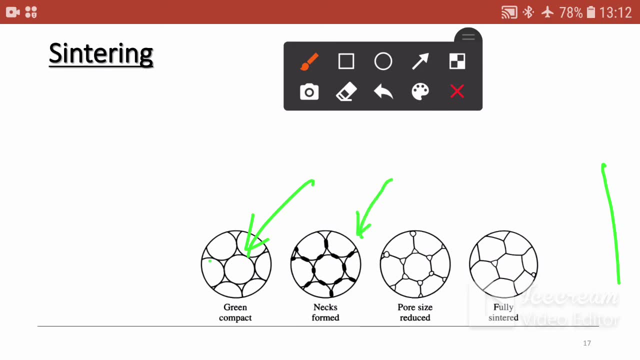 can see in this figure. so first, there is such type of mixture or such type of bonding is there in between particles. when we heat, what happens? this, this boundary, this, this is our grain, so this is outer, is boundary. so this grain boundaries starts melting, okay, and when it melts, it is. 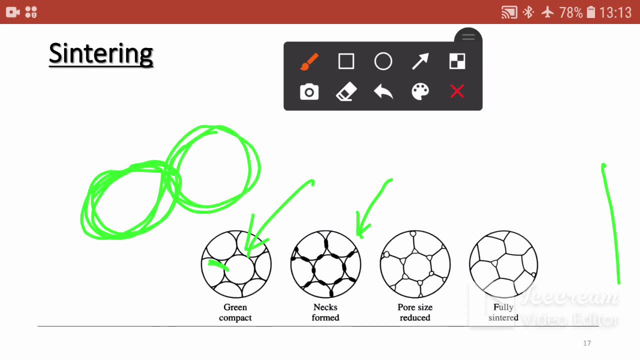 attached with another metal. okay, so it, it will also melt, this is also melt. so because of this boundary melting, see boundary, get melt and it will attach to another. okay, next, when it we, when we hit again, so there is more melting takes place and more strong bond between this particle one, two, three. 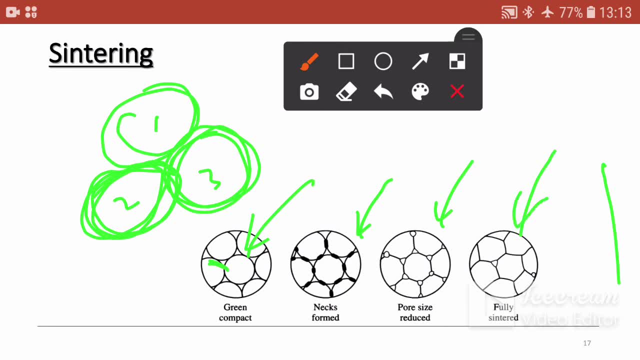 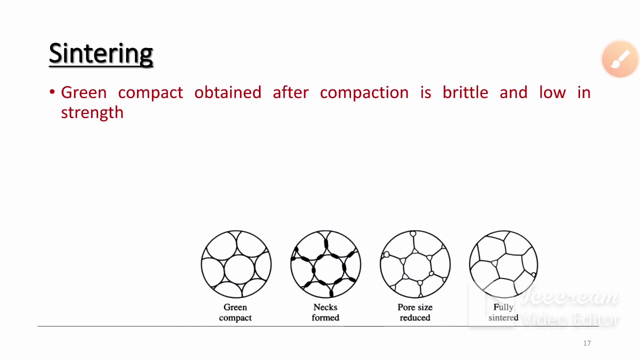 will be there, okay, and we are heating and also compressing. so because of heating and compression, you will get a very good bond, or strong bond in between this particles among the particles, okay. so these are attached very strongly. so this is the process of sintering. so green compact obtained after compaction is very brittle and low in strength. 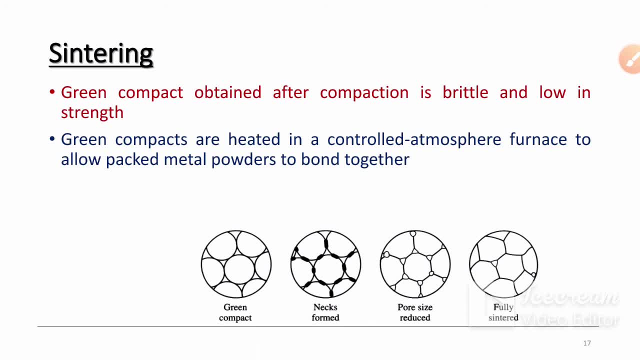 so green compact are heated in a controlled atmosphere furnace to allow pack metal powder to band bond together. so part are heated to 0.7 to 0.9 of melting temperature. okay, for example, melting temperature of this mixture is a thousand so you need to heat 0.7 to 0.9. 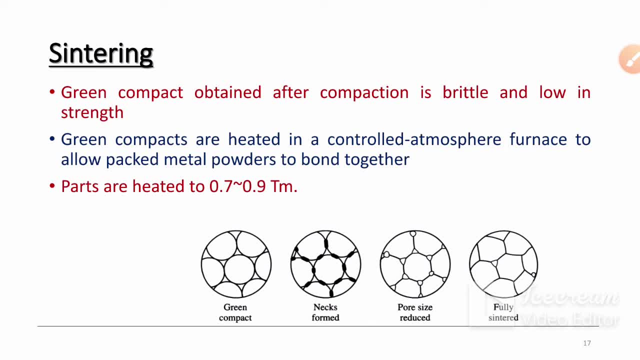 times of thousand. okay, this is sintering. so transformed, compacted mechanical bonds are too much stronger, metallic bonds okay. so only compaction will not give you a proper product. so after compaction, or compaction plus sintering will be simultaneously to get a strong metallic product. these are the three stages of 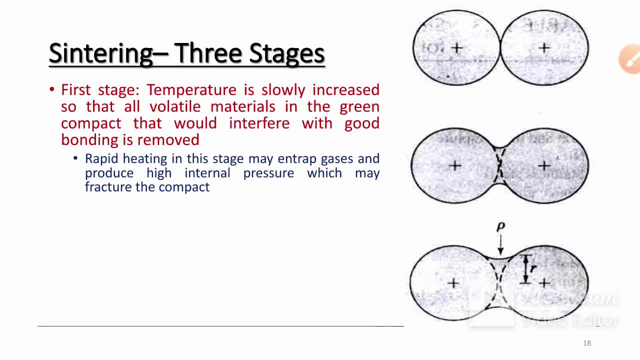 sintering already discussed. so first stage: temperature is slowly increased so that all the volatile material in the green compact that would interface the good bonding, is removed. then rapidly hitting this stage may interrupt the gases and produces the high internal pressure which may be fractured in compact. second stage is a high temperature stage. so third stage, sintered. 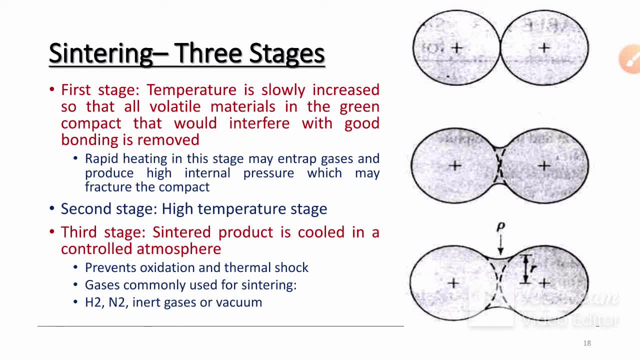 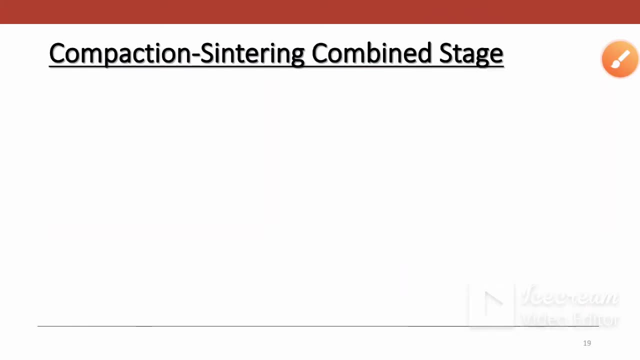 product is cooled in a controlled atmosphere. prevent oxidation and thermal shocks. gases commonly used for sintering: h2n2 and inert gases or vacuum. okay, so these are the three main steps. first is this metal, then heated, and third stage is cooled down. okay, then compaction, sintering, combined stage. so this is most. 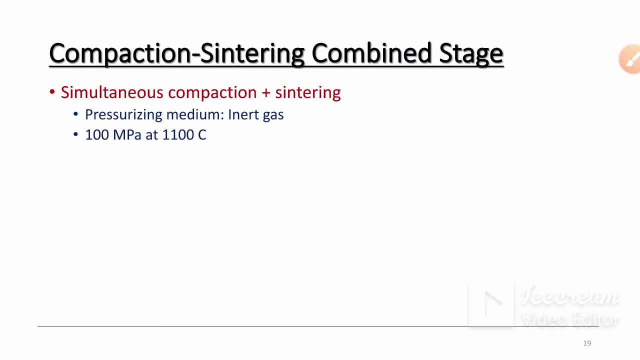 commonly used and sintering combined stage, so this is most commonly used and simultaneous compaction plus sintering is none. pressurized medium is inert gas and 100 megapascal pressure is used most commonly and at 1100 degree centigrade. 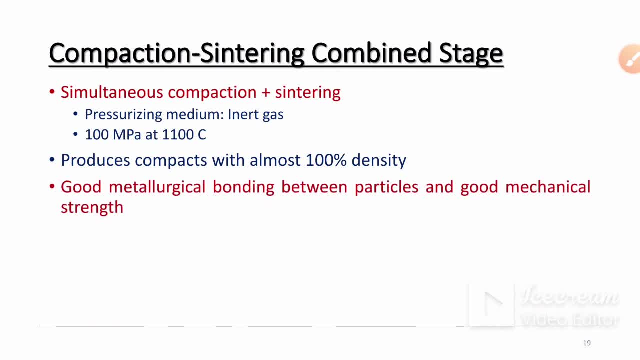 so produces compact with almost 100% density, good metallurgical bonding between particles and good mechanical strength. then uses are super alloys, components and aerospace industries. final testification: dis-application step of WC. cutting tools means tungsten, carbide tools and powder metallurgy tool steels. 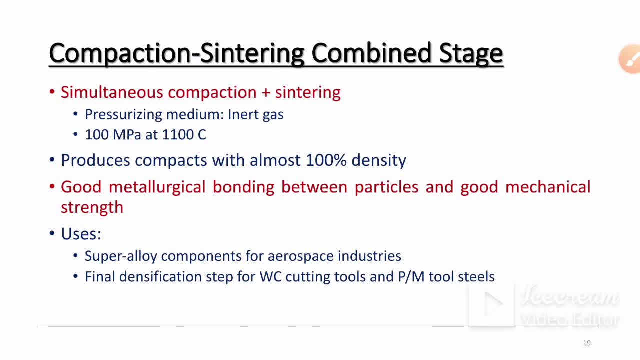 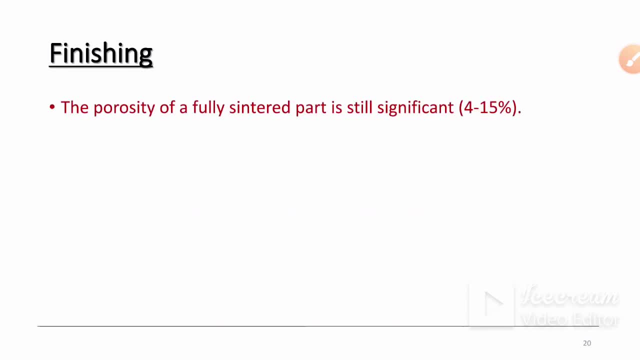 okay, so this is most common uses of compact sintering combined stage. next step is finishing steps. okay, now our product is ready, now is finishing. so the porosity of this fully sintered part is still significant. okay, when we sintered it then still, there is a porosity to 4 to 15 percent porosity is available or is. 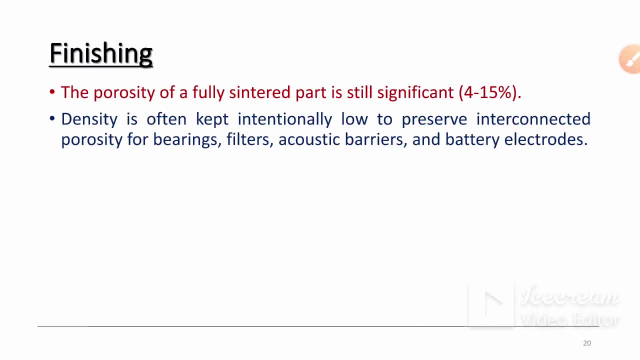 there. so densities often kept intentionally low to preserve the interconnection porosity, porosity for bearing filters, acoustic barriers and battery conductors. so most commonly, porosity is required when we use this metal in bearings. okay, so because of that porosity, or this lubricant will goes to the required- 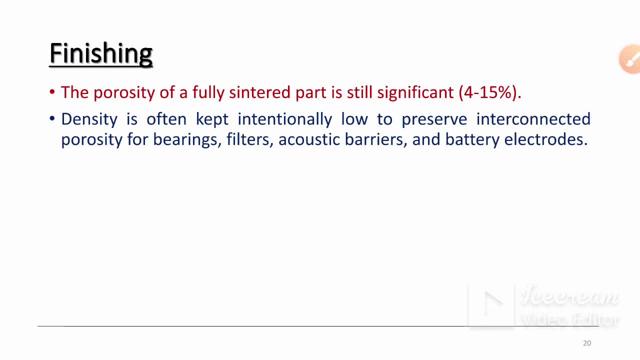 shape, required parts or required elements. and, however, to improve the properties, finishing process are needed. heat treatment, impregnation of heated oil and infiltration with metals or machining to tighter tolerance is the finishing processes. so first is heat treatment okay. so to improve some mechanical, thermal or chemical properties, heat treatment is often done. 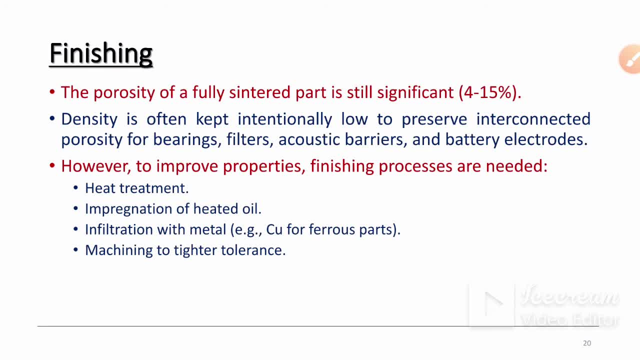 after completed the sintering process. so there is a heat treatment process after finished product. then impregnation of heated oil. so heated oil is added on these metal, okay, and when? so most commonly in bearing impregnated powder, metallurgy product is used. so infiltration with metals. so infiltration means we will melt the. 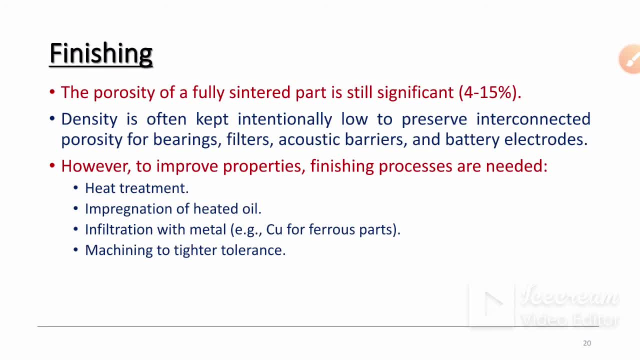 copper or any other materials, and we will pour this melted material on the porous product, porous powder, metal rich product. so when we add this heated or melted material on this porous product, then what will happen? the porosity of this metal, porosity of this product, reduces. okay, so there is liquid metal. fill up the